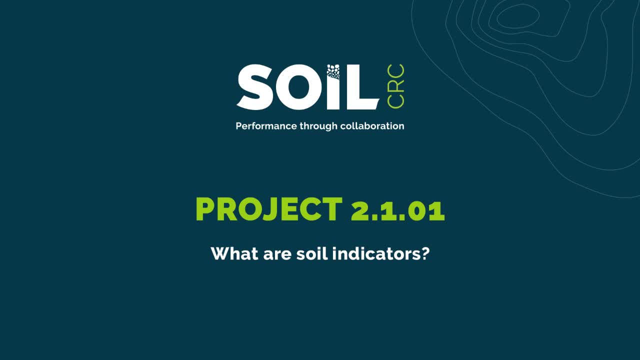 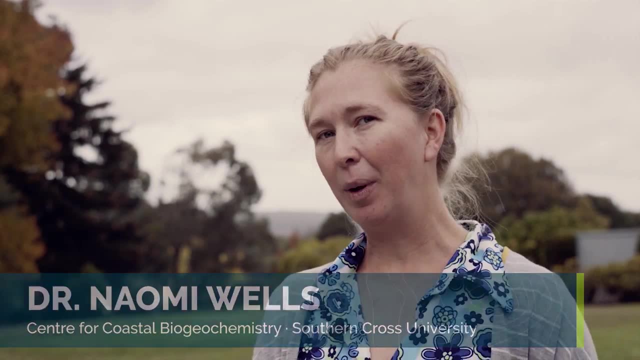 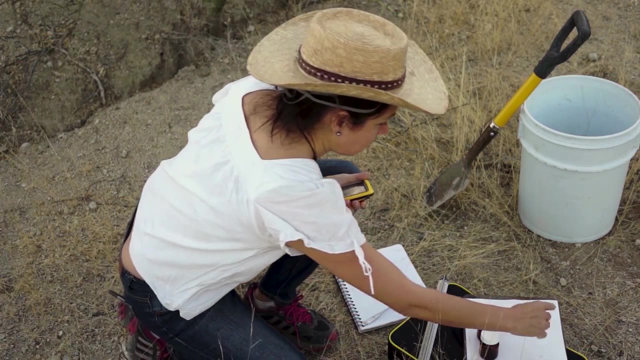 The goal of this project is to understand how, the kind of chemical or biological or physical health of soils, and whether we have things we as scientists can go out and measure in a field that will help farmers or end-users, land managers, whoever understand what's actually happening in. 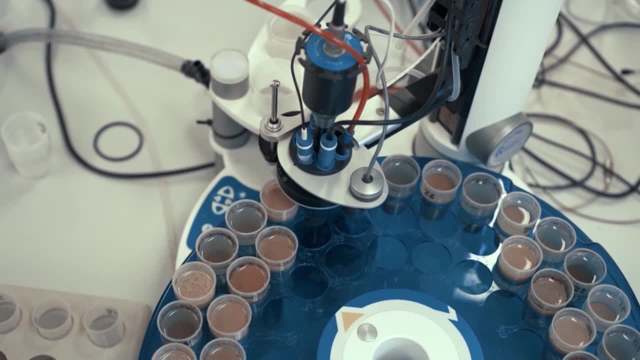 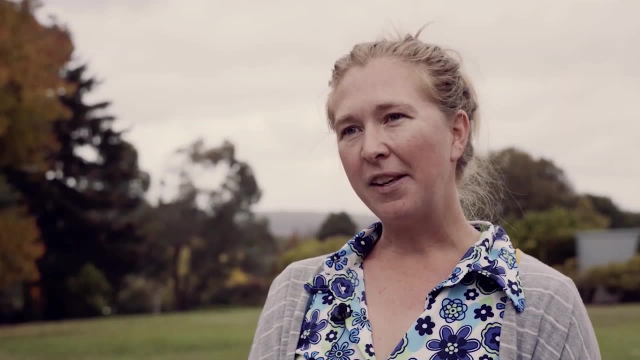 the soil. It's kind of one of those questions that seems super basic when a lay person maybe asks it, like obviously you just go and measure it and then you understand it. But the purpose of this project is to actually improve that, because a lot of the things that we measure in soil are 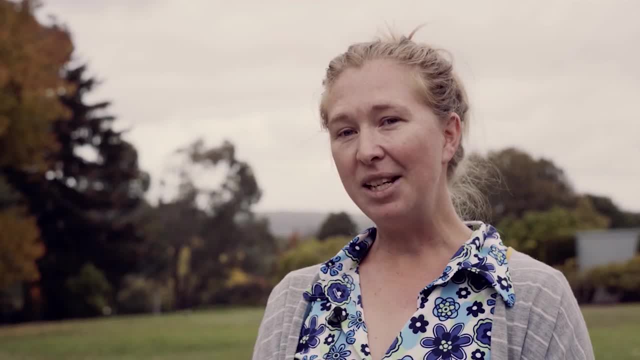 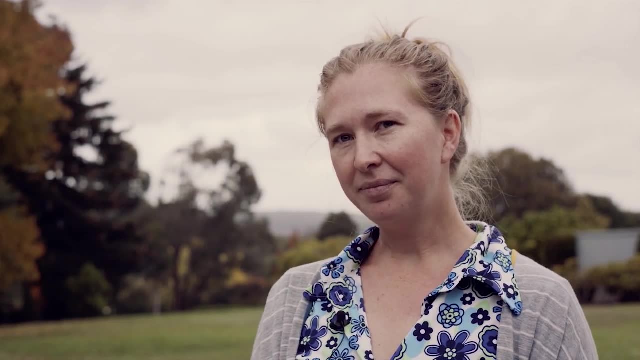 just based on maybe something 50 years ago that was easy to measure and maybe that means like a lot of the things we measure are just because that's the easiest to measure, not because it's the most accurate. People normally think of soil performance indicators for agriculture and for 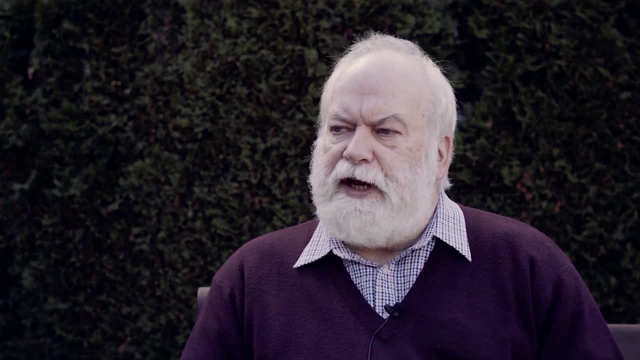 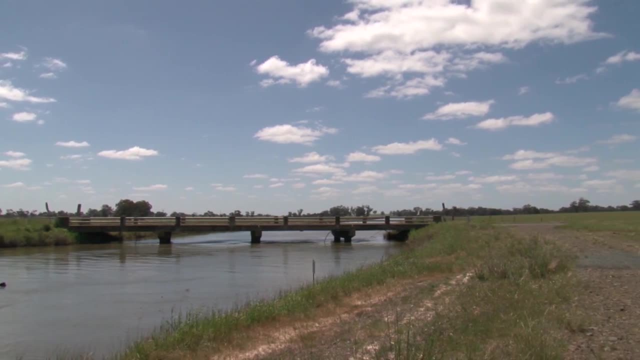 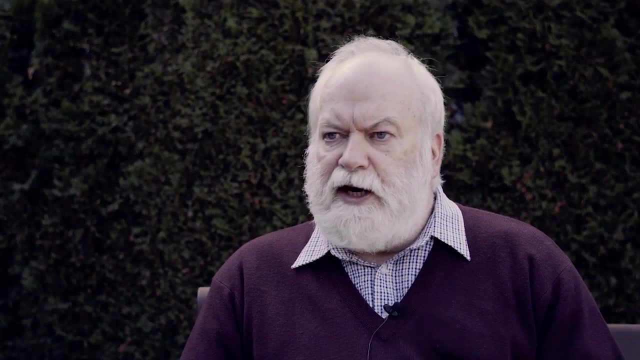 farming. but in actual fact, you know, indicators are broader than that, because indicators are also used to determine the value of the land or the state of environment reporting, or whether or not a soil has been misused or eroded away in the past, or something like that. So indicators are very 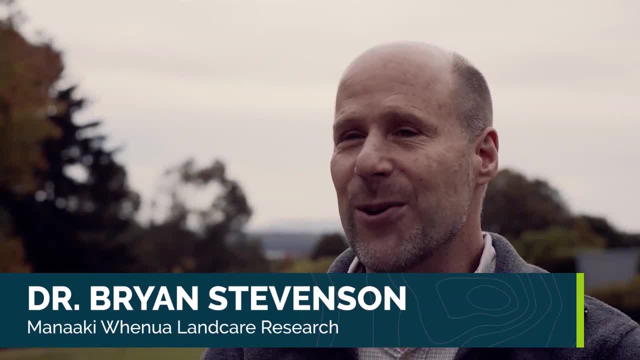 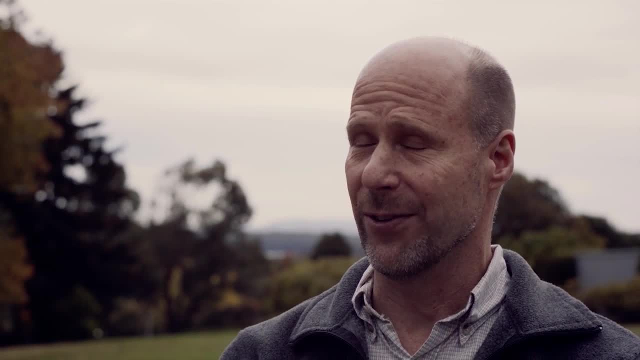 broad and very, very varied. So it's easy to to see what what poor soil health is, but it's difficult to measure what good soil health is, and that's why we need indicators. So the CRC is a very interesting and interesting project in terms of what it's about. So the CRC is a very 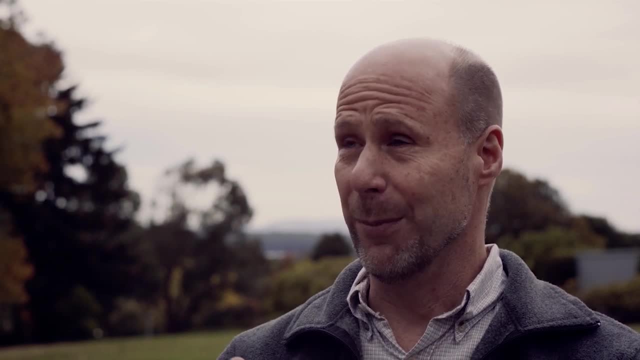 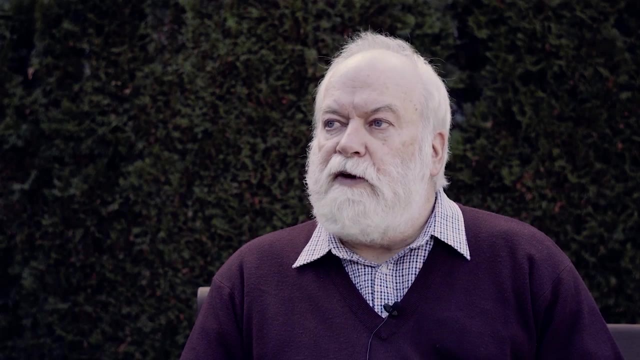 all about trying to find good indicators, indicators that really tell us something about the system. So when we're looking at this, at this particular scoping study, one of the things that we've learned about it is that there are lots of different indicators that people would like, so there are. 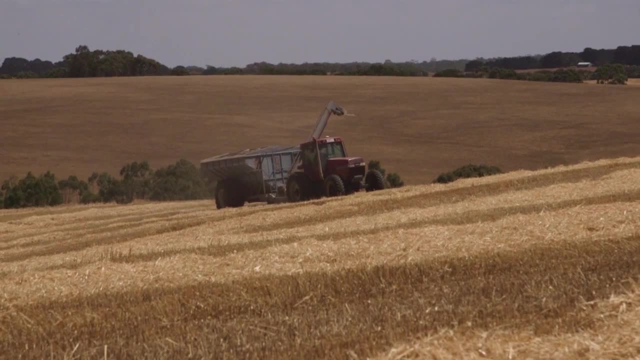 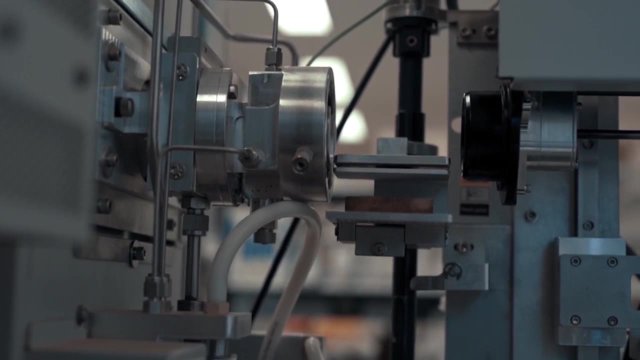 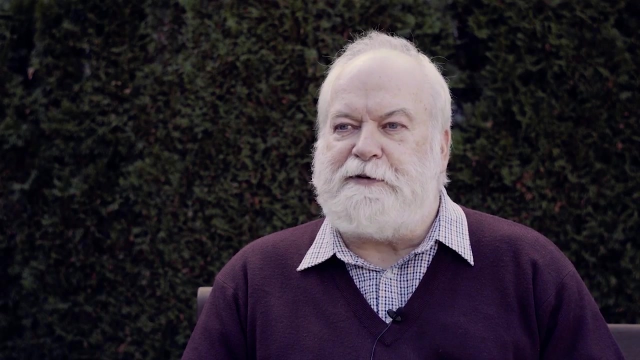 indicators that are sure a lot of indicators for farming, but they're also indicators for environmental indicators for finance, for banking, for, you know, Indigenous soil health assessment, for all sorts of different reasons that we didn't really think about beforehand.